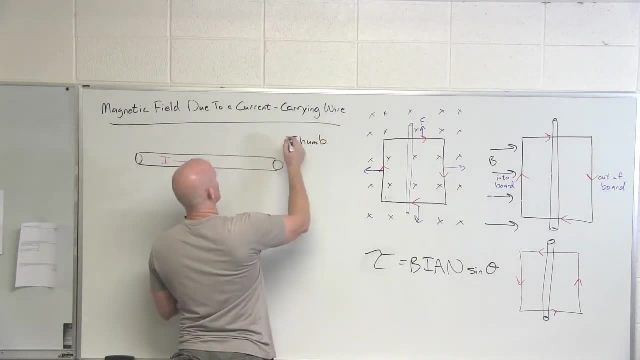 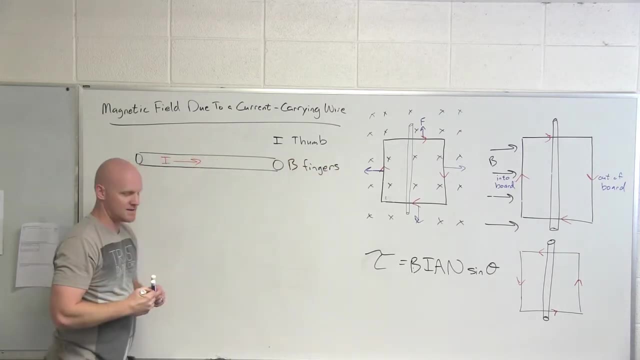 So you got your thumb, so, and that's where the current's going to point. And then you just got fingers, and that's where your magnetic field is going to point. And so what you do with this right-hand rule is you put your thumb in the direction of the current, and then your fingers curl around the wire to show you the direction of the magnetic field. And so in this case, it's just going around. Now let me ask you a question. Is this clockwise or counterclockwise? And be very careful before you answer that. It depends on if I'm looking at it from this side, or if I'm looking at it from this side. So we can't really say clockwise or counterclockwise with any kind of definitive answer here. So what we'll do instead is I'll tell you up above the wire, where does the magnetic field point? 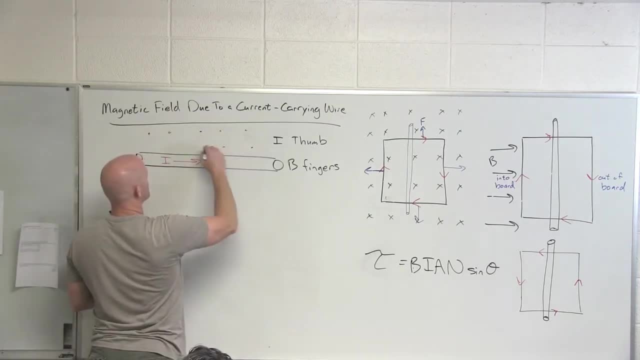 Out of the board in this case. If the current had been flowing to the left, it would have been into the board. 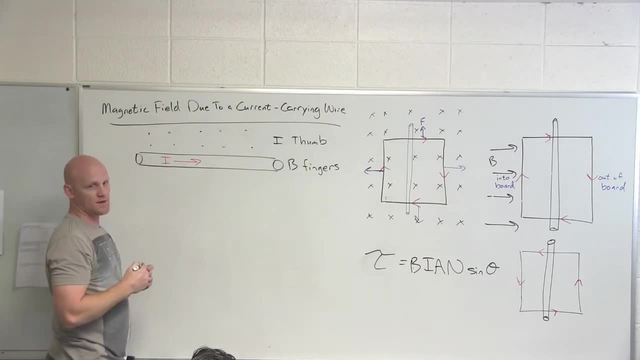 So where does the current, I'm sorry, where does the magnetic field point directly below the wire? 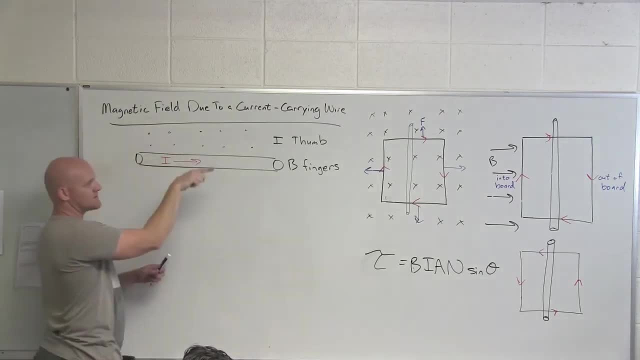 So again, thumb to the right, curls around the wire. So if it's going around the wire, think about this as the wire here. As it goes around, directly above the wire, the magnetic field would point directly out. Going around the wire, directly below it, it points directly in. Going around the wire again, magnetic field right in front of the wire would actually point down, and going around the other side, point up. And it's just going around. And around in a circle. Cool. 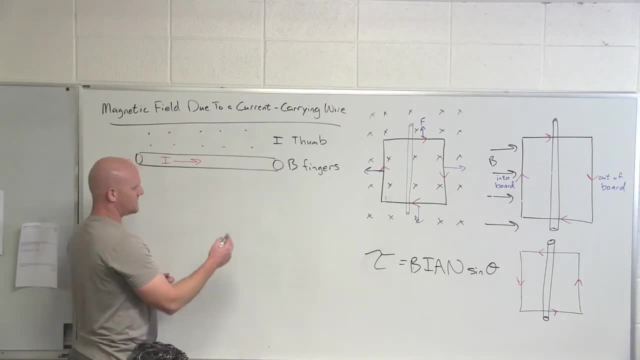 So think about it this way again. If you recall, going around in a circle, let's say we got circular motion here. 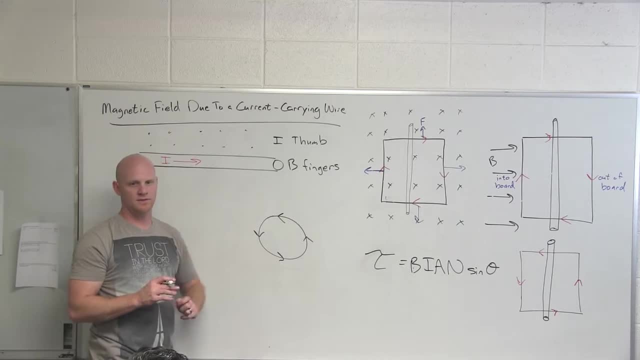 So let's say I got uniform circular motion, where does the acceleration always point? Towards the center of the circle for uniform circular motion. 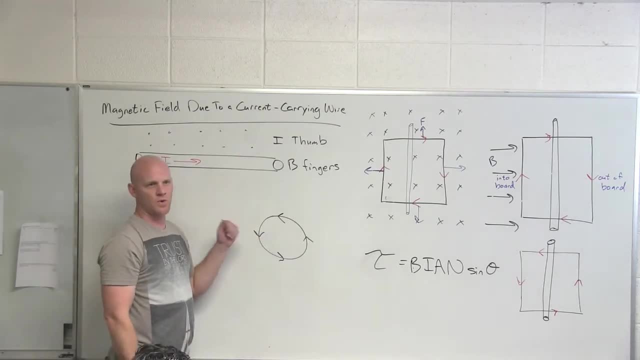 Centripetal acceleration, right? But where is your velocity point at any given point? Tangent to the circle, right? So at this point, it would point directly right, straight down, velocity to the, I'm sorry, directly left, directly right, and then straight up right here. 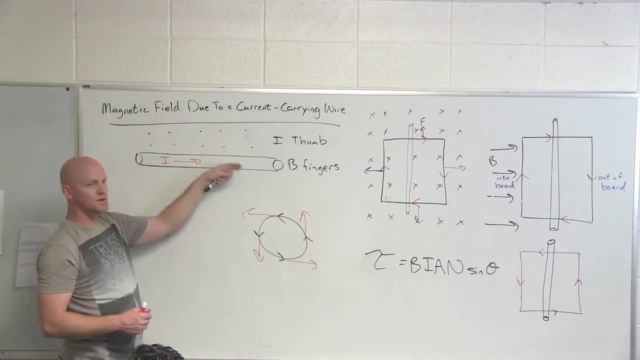 So it's always tangent. We have the same thing going on with our circle around here for that magnetic field. So as you go around the circle, so as you go around the circle of the wire, you can see what it's like. Now, like I said before, wouldn't it beSure 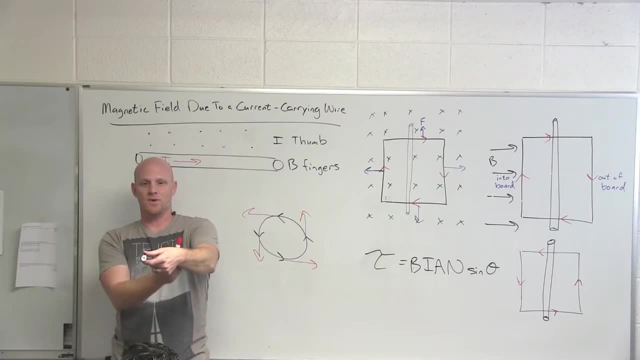 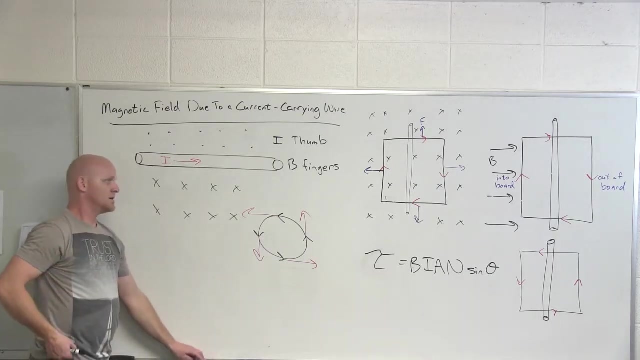 So it points towards your right. It points up. It points towards your left, and it points down going around the circle. And that's the direction of the magnetic field going around. So now, in orienting it this way, your magnetic field points into the board, up, out of the board, down, and just keeps going around. But it goes around radially, and you just need to put your thumb in the direction of that current to find out, does it go around this way, or does it go around this way? and indeed in this case it goes around this way into the board so again as you curl around where do you intersect the area right above the wire coming out of the board where my fingers would point whereas coming back around to the other side as we go around to the other side they would point into the board so again keep that let's make the red one the wire this time because it matches our current there so if your magnetic field is going around this way then up above it points out and down below it points into the board cool so and so again where does it point out in front of the wire out here out in front of the board where would that magnetic field point down and behind the board up that's how it works cool so now this is gonna get tricky because now we can draw the 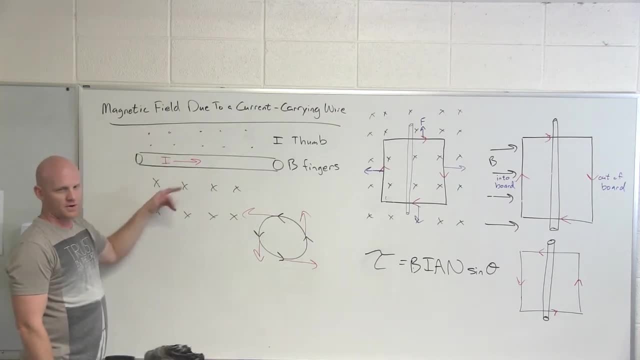 magnetic field that this wire is going to be pointing out to the other side of the board but earlier we just showed the magnetic field that was external this that he felt and so students often get confused so are we drawing the one he's causing or the one he's feeling and stuff like that well right now we're doing the one he's causing that is radially around him all the way around and the closer you are to him the bigger it is so we shouldn't be surprised to see that the strength of your magnetic field is inversely proportional to the distance of center of gravity so we're going to draw the magnetic field that's separation the distance away from the wire cool the greater the current the greater the magnetic field so and there's this lovely new constant permittivity of free space 4 pi times 10 to the minus 7 it's on your handout just another constant to get thrown out there and we're talking about magnetism cool notice look at your equation here so with this right-hand rule how many things did we have to define just two why didn't we have a third one where's no force as part of this this is nothing to do with force in and of itself anyways so it is just the strength of magnetic field due to a current in a wire cool so that's why there's only two things to define but this is a little different than the ones we've had but at least 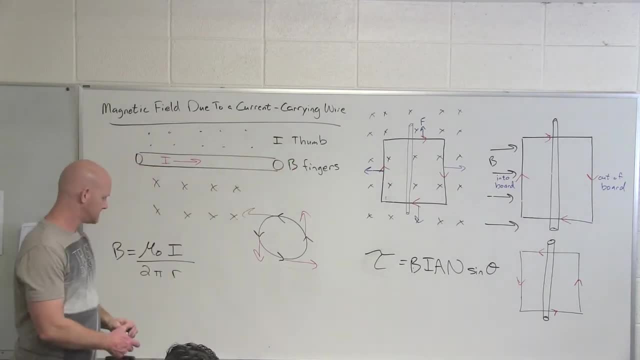 your fingers and your thumb are still defined in the same fashion all right so we've got two wires 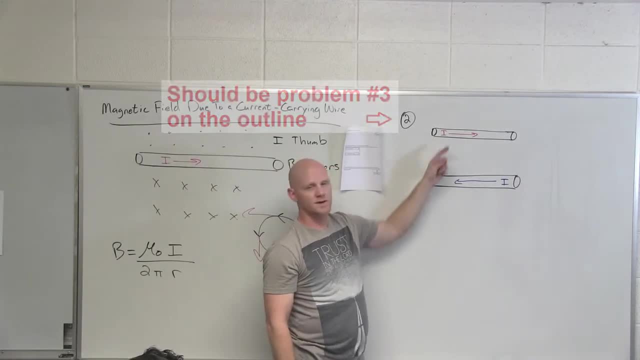 here and these wires are parallel but their currents point in opposite directions so question number two says 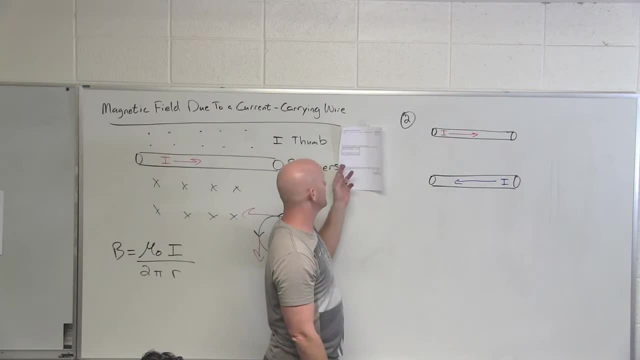 is the force between the following two wires attractive or repulsive and what would be the effect of doubling the current in both wires on the force between the two wires so let's look at this for a minute so in this case this is tricky because both wires cause a magnetic field both cause you know a magnetic field due to exactly what we just said but because they both cause a magnetic field then each has the opportunity to feel the other's magnetic field so we're going to look at the magnetic field now if we talked about the magnetic field that each cause what's our equation cool but if we talk about the force that they feel due to the other's magnetic field what's our equation yeah bil sine theta so this is the magnetic field that one causes but this is the force it feels due to the magnetic field the other one's causing so on and so forth so keep that in mind so if we look at this we want to find out is this an attractive force or repulsive force so in this case either you know both wires are repelled or they're both attracted to each other we're just going to figure out the directions of the forces but we got to apply two right hand rules and this 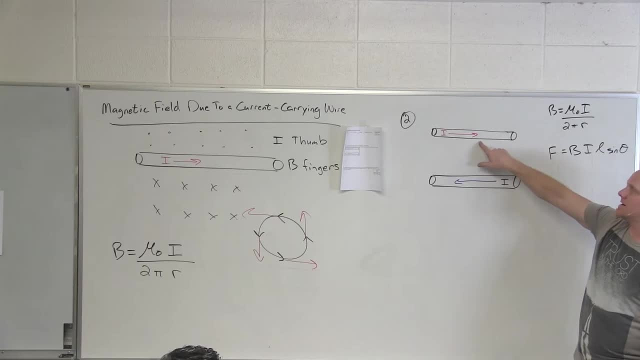 is super confusing the first time you do it so first let's look at the magnetic field that the red wire causes so in this case that's the one we already set up right over here right so the red current here go into the right has the magnetic field going over here we've got two direct forces around the wire. Where would that magnetic field point up here? So out of the period, out of the board. Yep. Towards you. So where would it point out in front of the wire down behind the wire up? Where would it point right down here in the plane of the board into the page? So that's what I'm going to do here. I don't really care where it pointed and all those other instances. 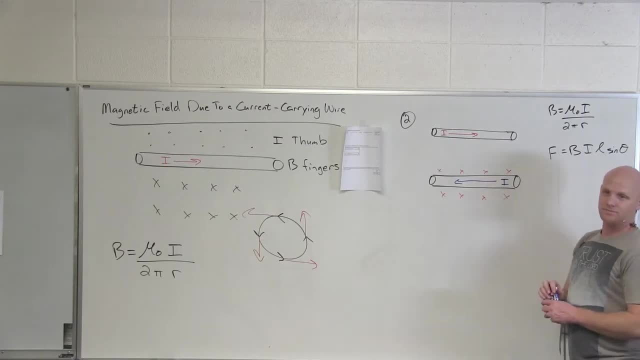 I just need to know exactly where it points right where this wire is. Okay. So if we look at that, then I can then, so that was this kind of look at the right hand rule that went with this 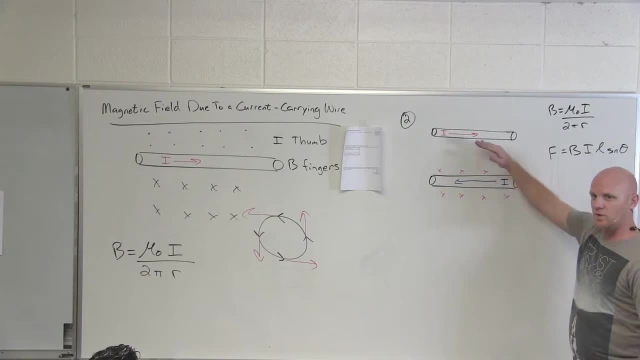 Well notice everywhere down here in the plane of the board, it points in, it gets weaker the further you get away and everywhere up here it points out of the board. So, and everywhere out in front of it, the further you get away, it always points down and you know, so on and so forth. Cool. I just wanted you to show that, you know, everything below him at all points in and the plane of the board here. 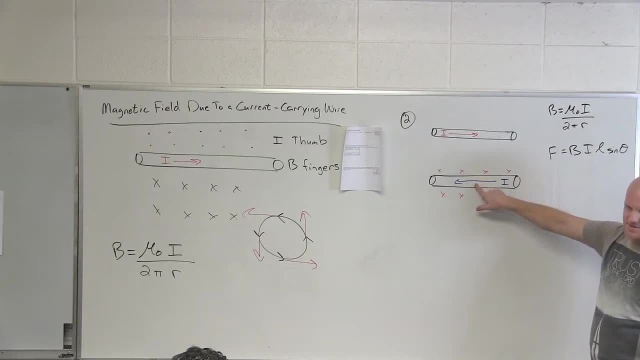 Cool. So then the question is, what is the direction of the force on this wire, this equation now? 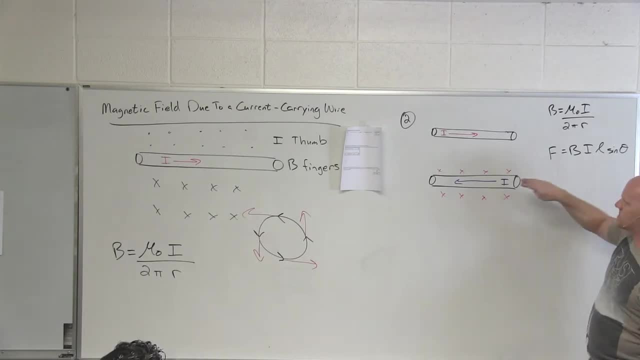 So what's our right hand rule for this fingers go into the board thumb in the direction of the current, 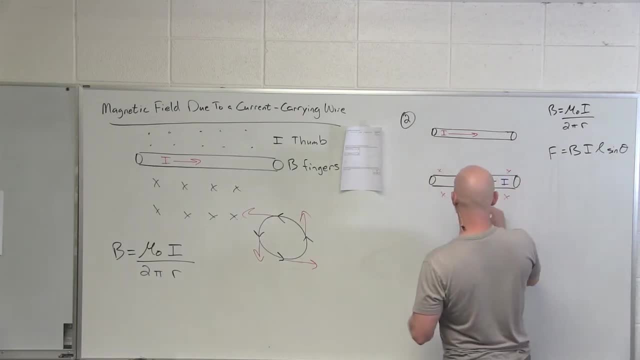 where's the force and the force it feels is indeed a downward force. Cool. Two right hand rules to figure that out. 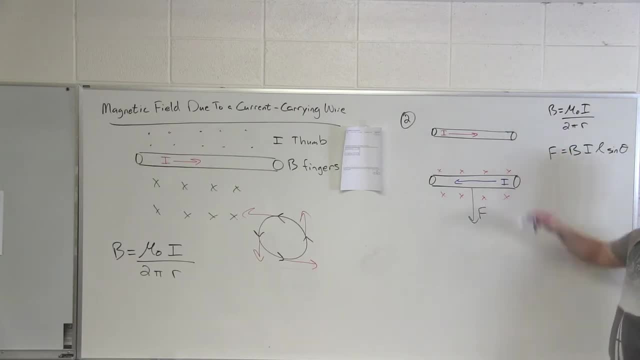 Now let's do the same thing for the other wire. So now this wire is feeling a force because the blue current is causing a 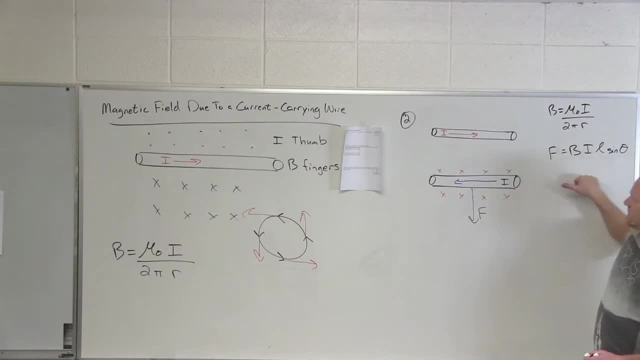 magnetic field. Now the blue current here, it's current points to the left and you curl your fingers around. 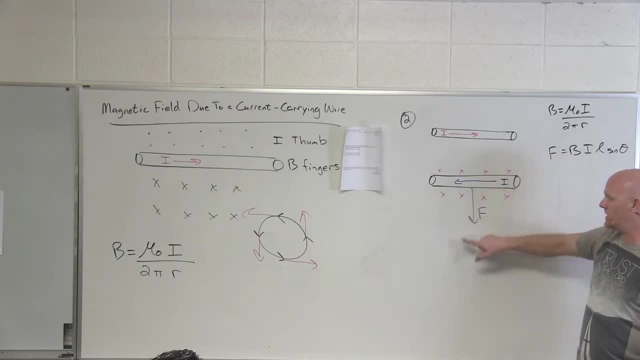 So, and where would the magnetic field caused by this wire point way down here? So out of the board and I don't care, right? Where would it point right out in front of the wire? 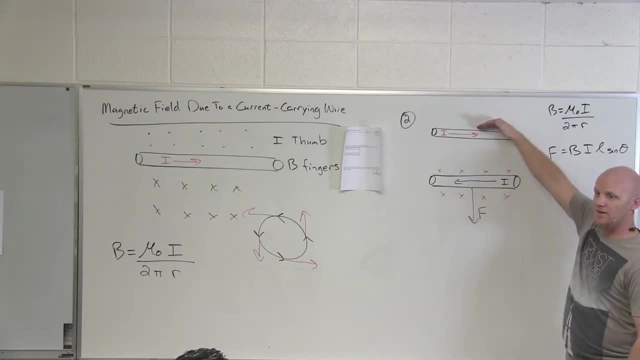 Oh, so where would it point up here where this other wire is located? 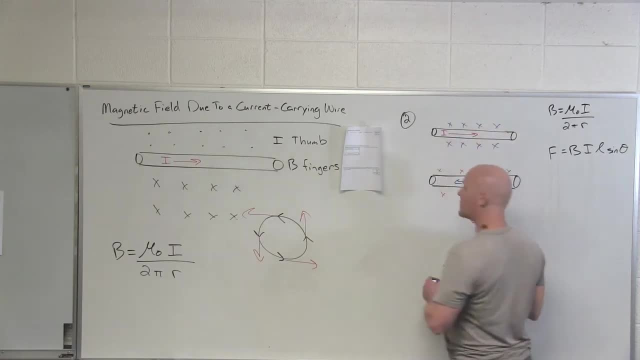 Good into the board everywhere up here in the plane. And that's the only one I really cared about. We just had to get there. 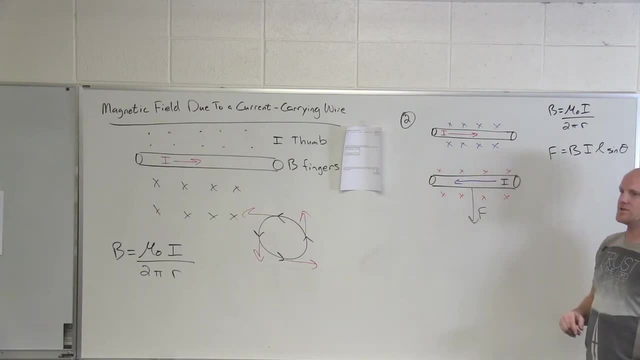 Cool. So now I look at the force. This wire is going to feel due to that magnetic field caused by the other wire or the current, the other wire. And again, I go back to this equation and his right hand rule. 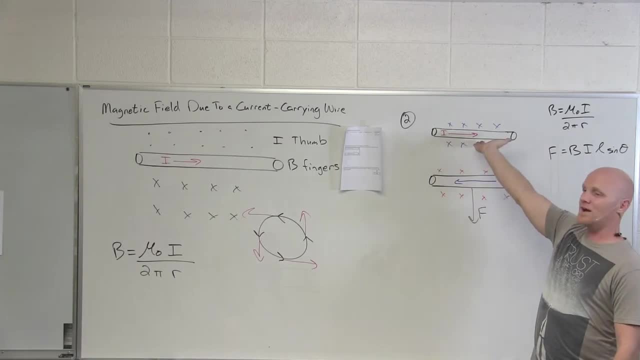 And so in this case, fingers go in currents going to the right. And where's the force up? 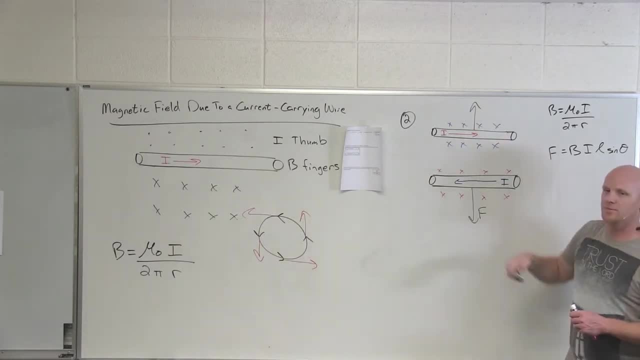 And so it turns out what kind of force attraction repulsive here, but it's a repulsive force. So it turns out if you have two parallel wires, their current needs to move. It's in the same direction for it to be an attractive force. And we just learned that when it's an opposite directions, it's a repulsive force. Cool. But that's how this works. 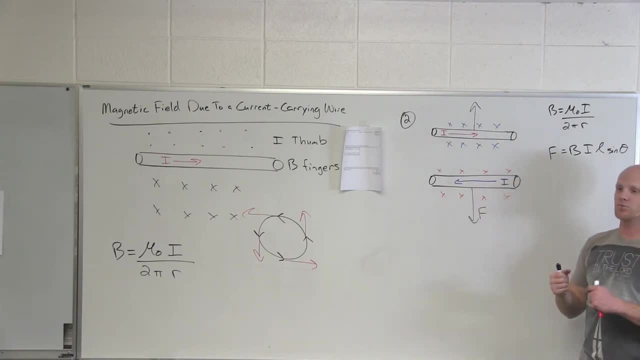 So notice that each wire you've got two different sets of right-hand rules to apply, and it's real easy to get tripped up on what you're doing. 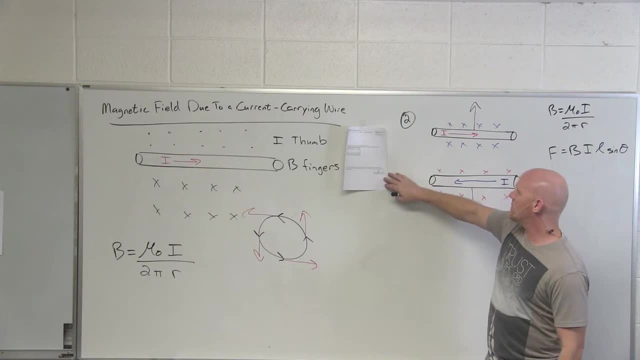 So we look at the second half of that equation. It says, so what would be the effect of doubling the current in both wires on the force between the two wires? 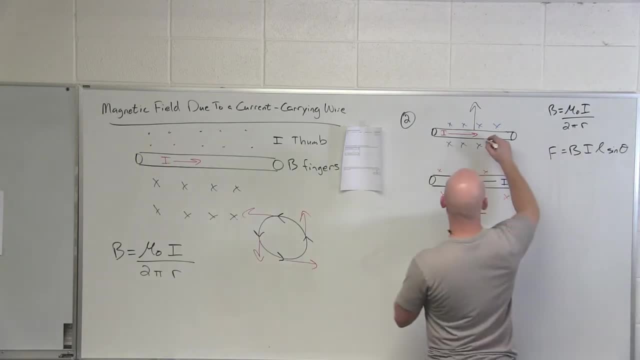 So let's just pretend for a minute that this wire had a current of 20. 20 amps. And this wire has a current of 10 amps, 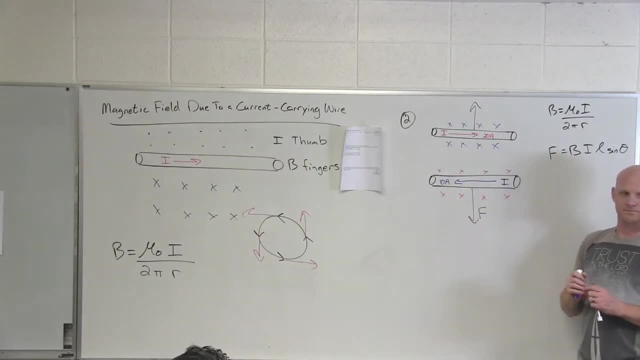 which wire feels a bigger force. That was a trick question. Just so you know. 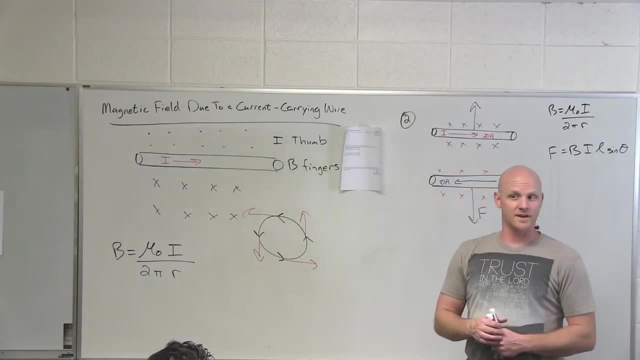 So if I push you, Chris, what did you simultaneously do back to me? According to Newton's third law. That's right. 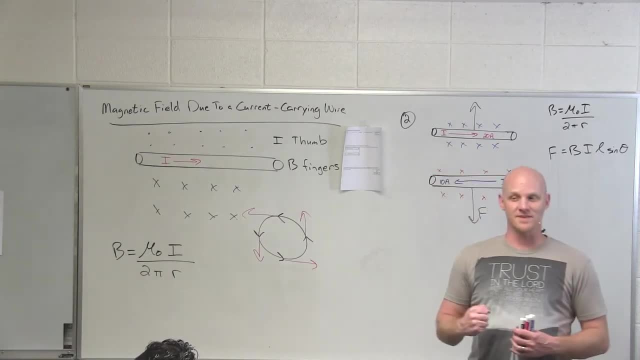 So I really appreciate it. If your face would quit hitting my fist, I'd appreciate that. So, but there's always an equal and opposite force. 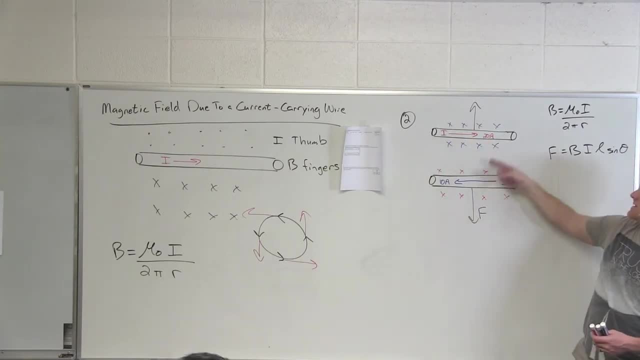 In this case, it's an equal and opposite force, regardless of the actual currents between the two wires and stuff like that. 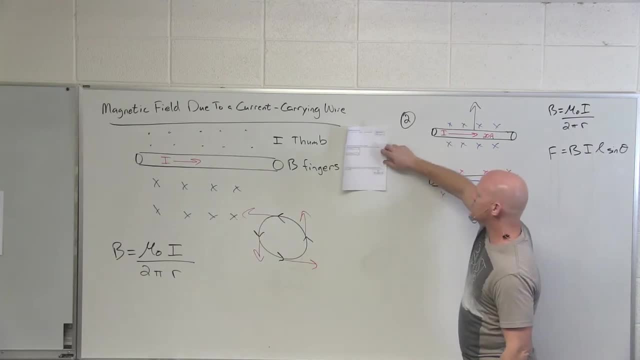 So that's the first part. So that's kind of an extra question I asked you there, but what would be the effect of doubling the current in both wires on the force they feel? So if I look, if I double the current, the wire, what's going to happen to that force and doubling the current in both wires. So I'll make this 40 amps and 20 amps. What would that do to the force? They feel so it would multiply by four. 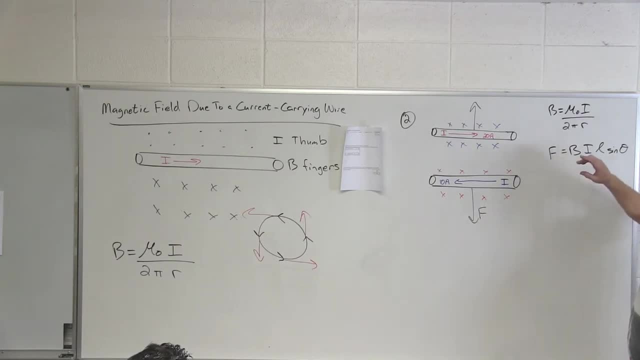 That is right. So let's look at this. So if you look, if I double the current in one of the wires, what does that do to the magnetic field? It, it causes, it doubles it. And that magnetic field peers right here, but I'm also doubling the current in the other wire. And so both of these are doubled and the force is quadrupled. Very cool with that. Cool. 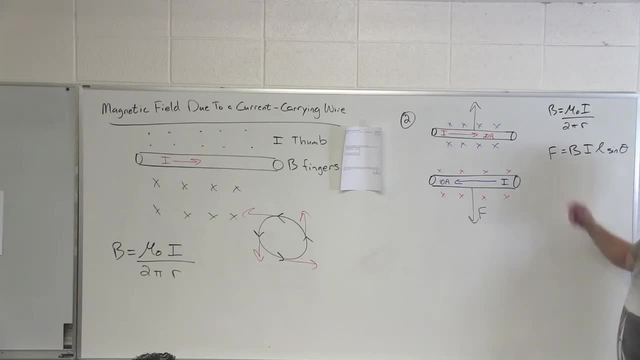 So it's really easy to get focused only on this equation that deals with force and be like, Oh, you double the current. Only one of them shows up. 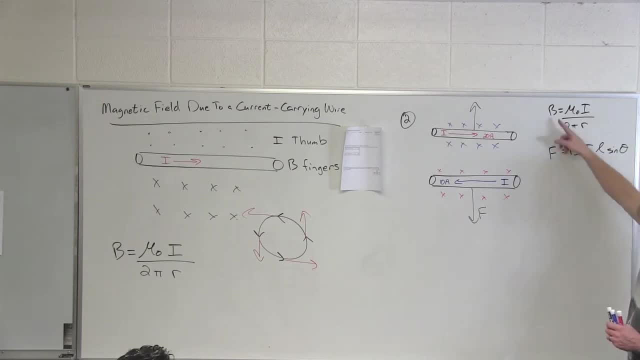 So you double the force. Well, they technically both show up. It's just the other one shows up inside of the magnetic field created by the other wire. 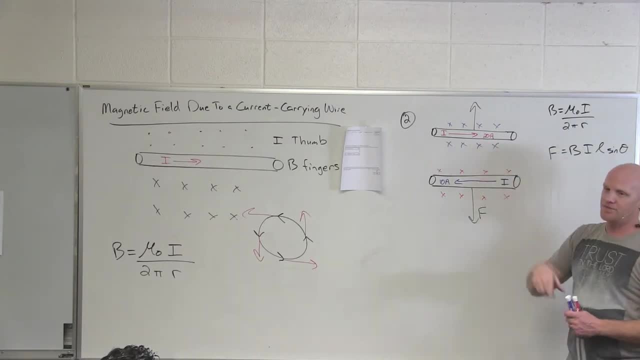 So if you double the current in both wires, what happens to the force they feel? And in this case, it quadruples. 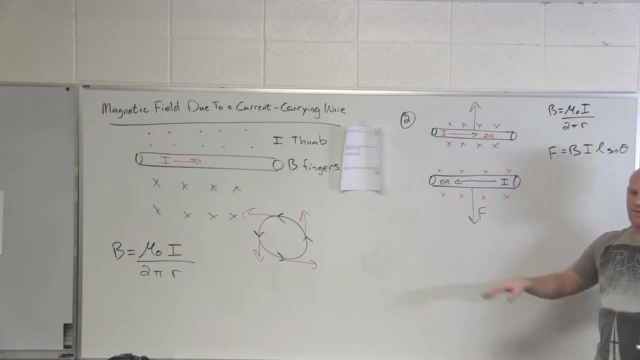 So the one before I was just saying who feels a bigger force and that was where they were equal and opposite equal magnitude, opposite direction. Clark. 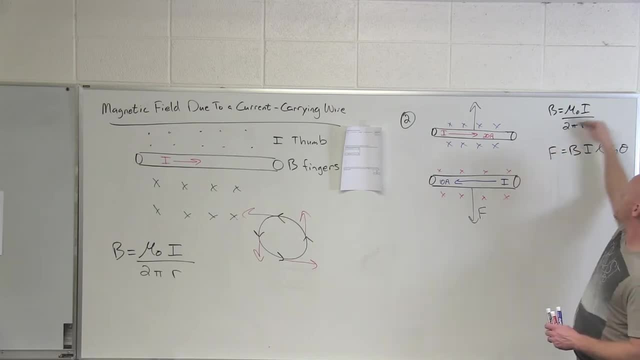 So your thumb just has to go with the current. So you're talking about for the right hand rule in this guy. Yep. 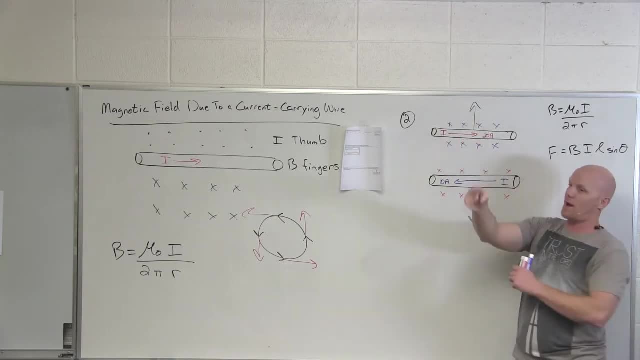 If your thumb goes with the current, your fingers can only curl one way. If you can curl them the other way, props to you. So, and you're screwed on this anyways. So, but in this case, thumb goes this way. Then your fingers have to curl that way. 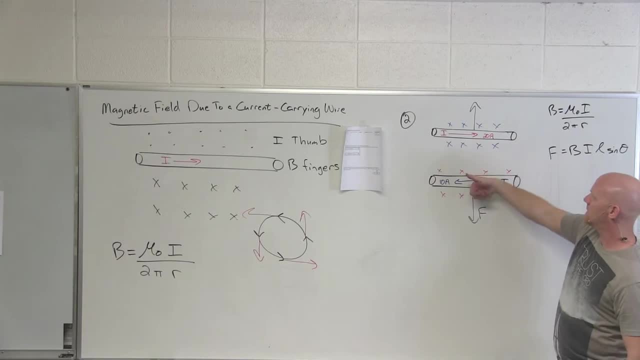 So out of the board down here into the board up here, up out in front of the wire, down behind the wire. The only place I cared about where his magnetic field he was causing was happening was at the other wires location and up there it's going into the board down here. It's going out of the board, but there's nothing here to feel it. So I didn't really care. Write it. Cool. 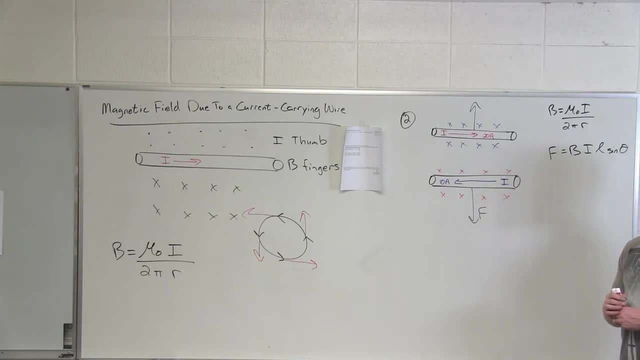 Could you just use the one where I can roll twice? So for the top wire, it would be going into the board on the bottom or the bottom wire. It would be going into the board on the top. So you would have both of them. 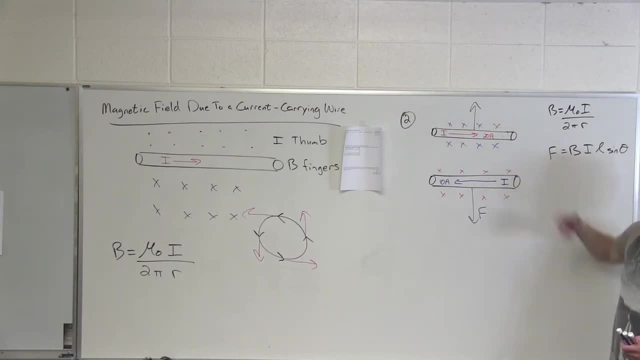 So you, and we found out that exactly fact, you know, into the board at both locations was true. So, and because the currents pointed opposite directions, they were going to feel a force and opposite directions, but we still had to figure out, was it up and down or down? And up to still figure out if it was attractive or repulsive. So we still had to apply that other right hand rule. 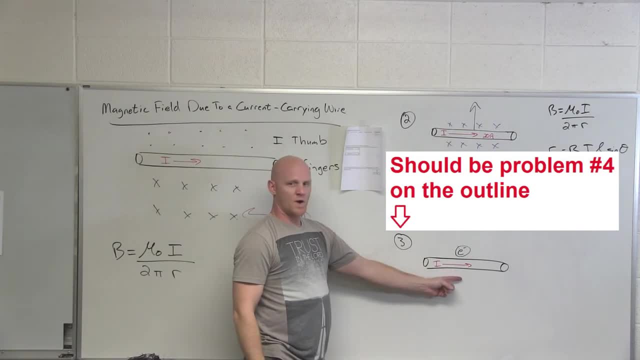 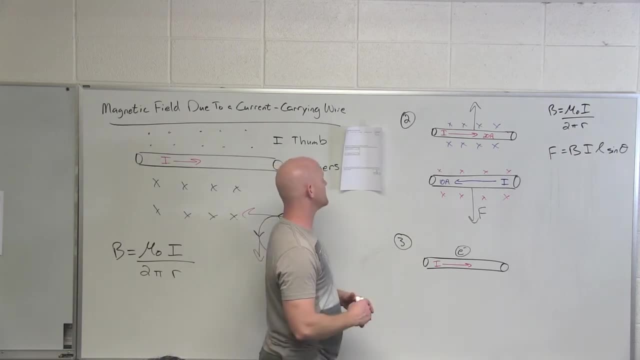 All right. Question number three, we've an electron right above this wire. So this wire has a current pointing to the right. So in the question says the electron depicted below is directly above the wire and is experiencing a force in the downward direction. Do the magnetic field created by the current, the wire, what is the direction of the electrons velocity velocity at this moment? So this thing is this electron is feeling a force. Pointing down a magnetic force pointing down as the question is, well, okay, what velocity does it, what's the direction of its velocity at this point? Okay. So right hand rule, what needs to point towards the, what's usually the force, the palm, since this is a negative charge, we'll be thinking that it's the opposite though. So we'll keep that in mind. 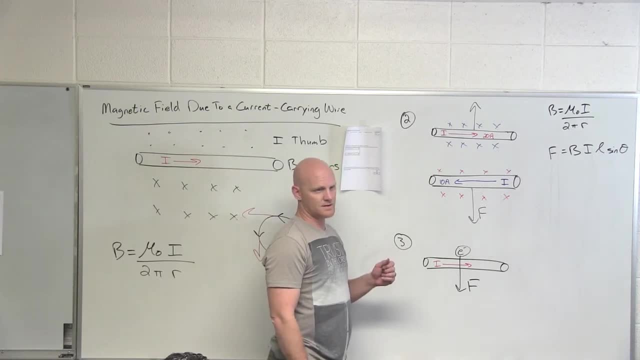 Current is going to match up with your thumb and magnetic field. Where's the magnetic field point at that location? 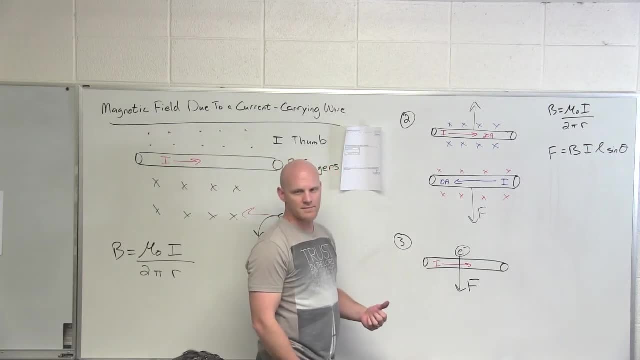 So that's another two right-hand rules in the same problem kind of thing. So first right-hand rule again deals with this guy. And at this location with the current point of the right, where's the magnetic field point right where that electron is located? Good. Out of the board everywhere up there. It's a really pathetic circles. Okay, cool. 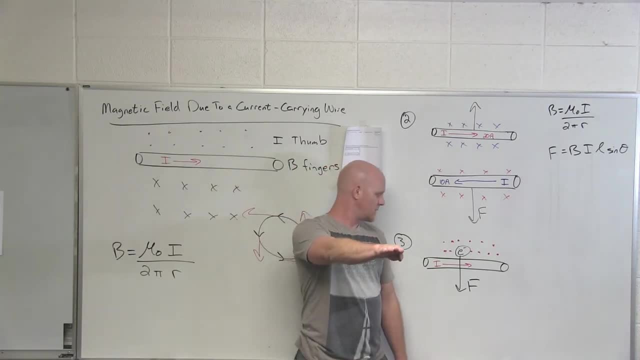 Now that I know that the magnetic field points that direction, I'll put my fingers. Out of the board, I'll put my thumb to the right with the current. 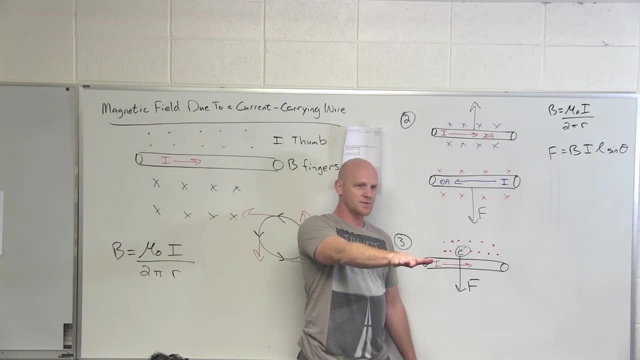 And if this were a positive charge, the force it fells would be down. Oh, what am I getting wrong now?